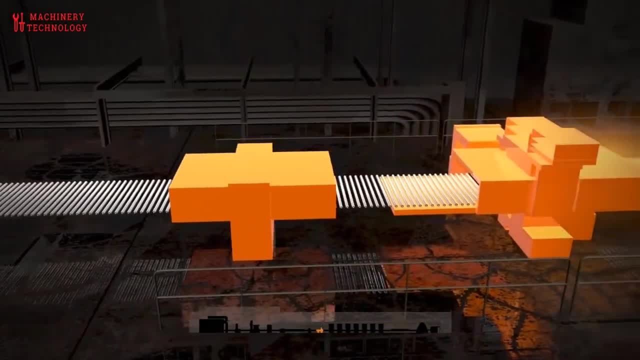 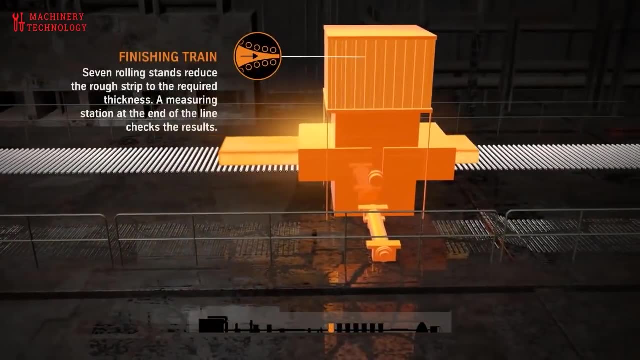 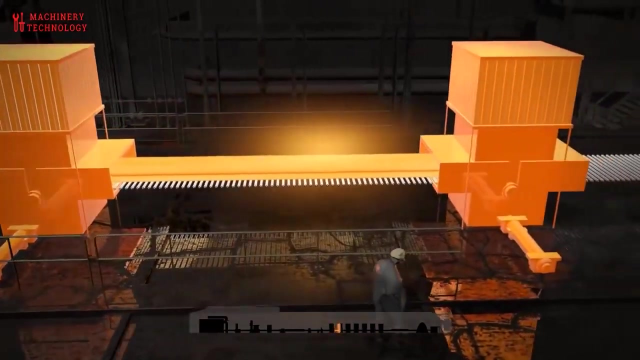 in which a metal stock is passed between two rolls in order to reduce the thickness and get a uniform thickness. Rolling is the initial process of a steel product's manufacturing, such as a structure of steel and coils. Rolling mills can process steel quickly and convert semi-finished, costing products, including ingots, blooms, fillets or slabs, into finishing. 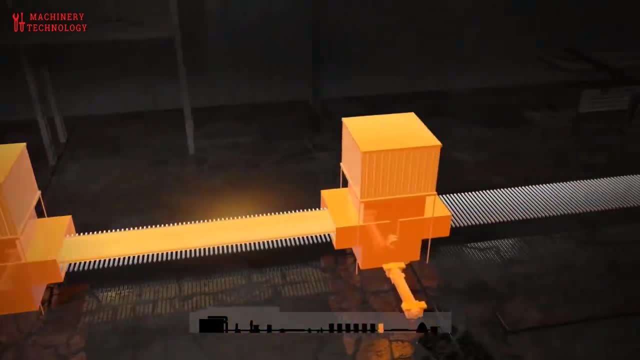 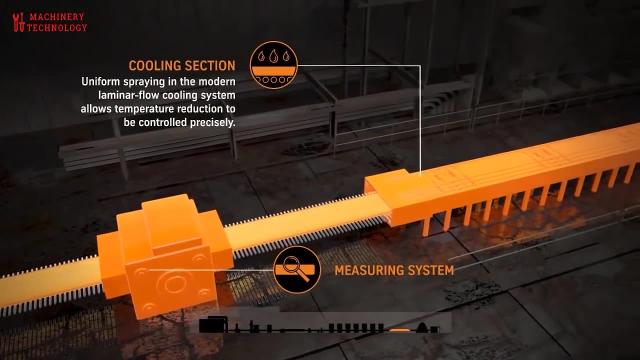 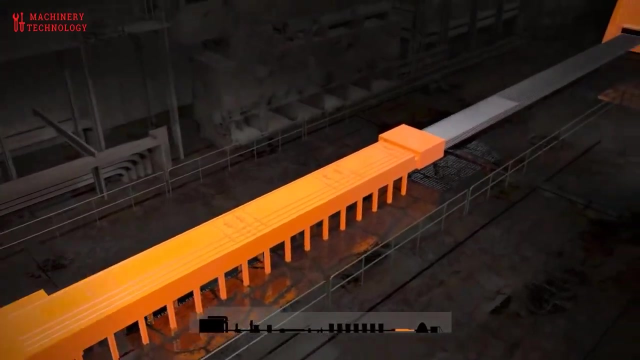 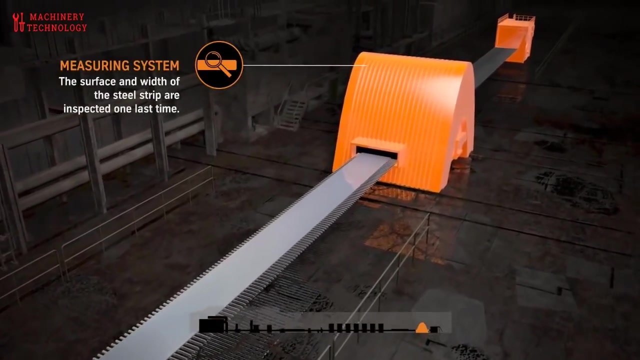 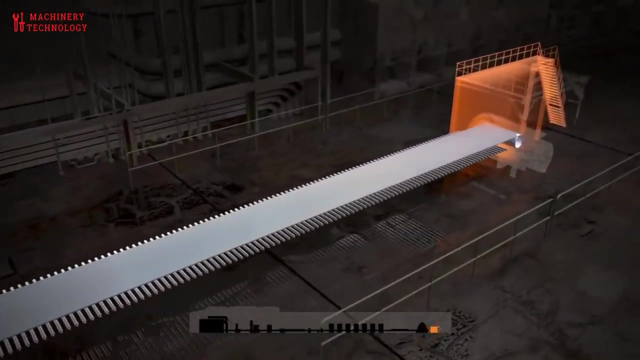 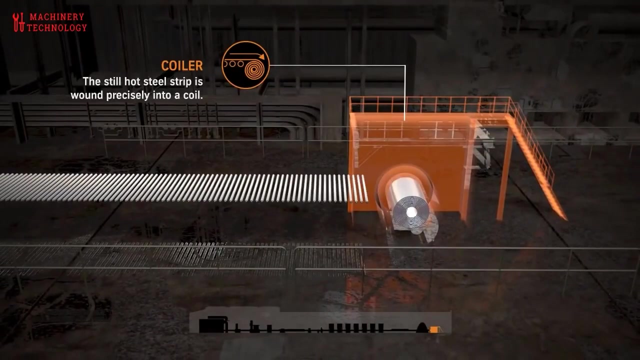 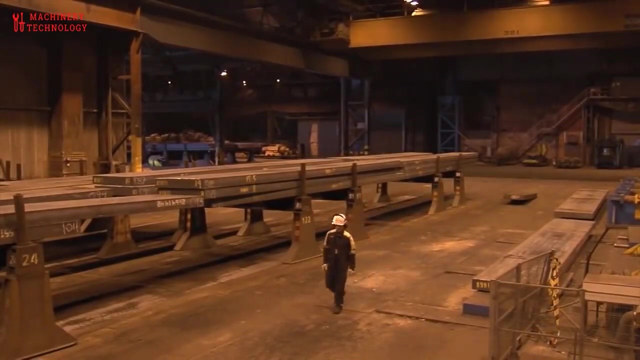 products like beams, bars or coils, etc. Hot-rolled steel is a steel that had rolled past a very high temperature, Approximately more than 2,000 degrees Fahrenheit, which is above the reclamation temperature for the most steel types. Hot-rolled steel is a steel that has rolled past a very high temperature. 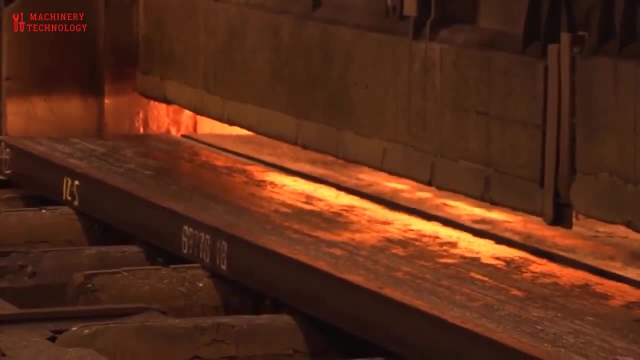 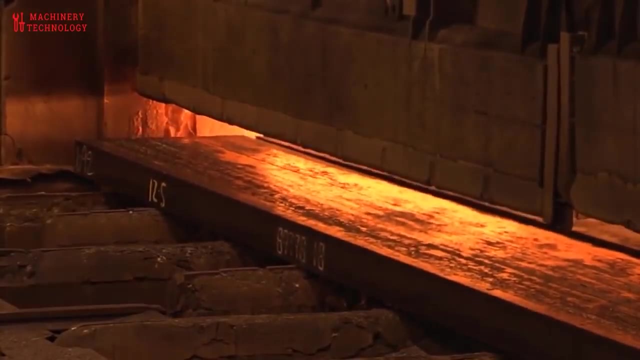 When a steel-like steamer is connected with a coil, its heat resistance can be increased to a maximum of 85% in 5 minutes. This difference is actually limited because of the heat retention. If the steamer is remembered as the most important part of a gas-operated welding process, it is the core of its performance. 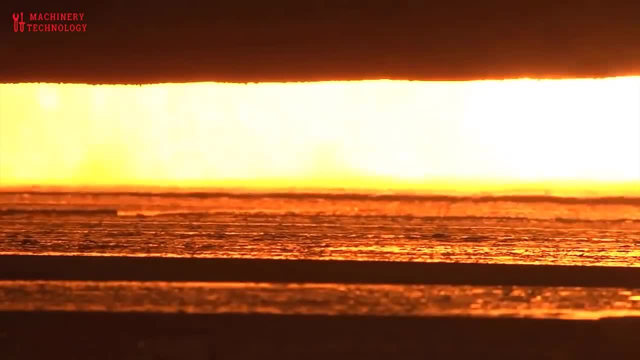 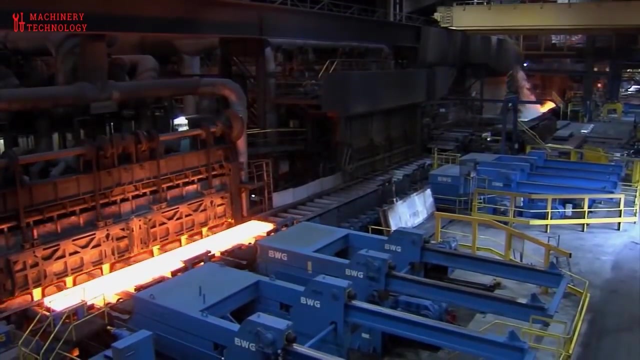 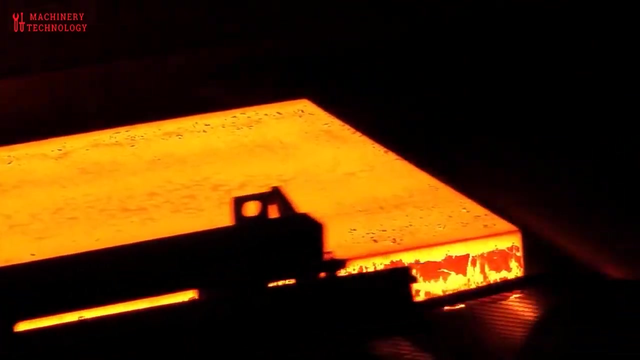 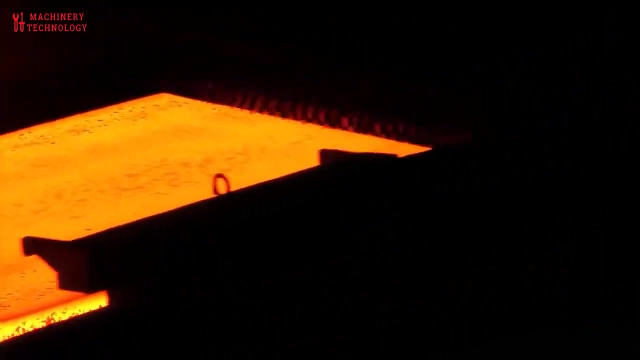 The head, gives a steel workable starting form and makes it easier to shape. Hot rolling starts with a large, long steel called billet, which is heated and sent to a large roll to flatten. Then it is passed in a series of rolls, keeping its high temperature until reaching the final. 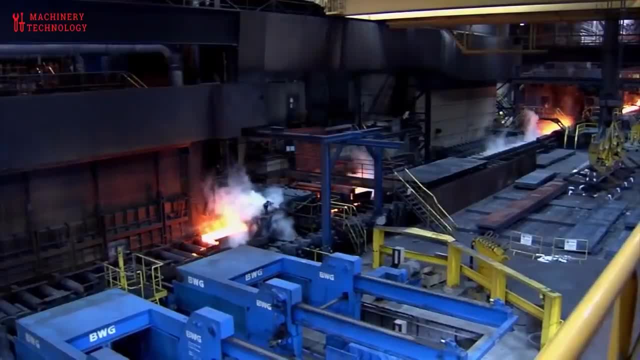 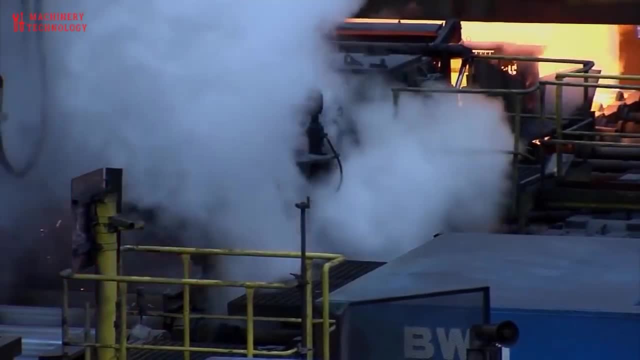 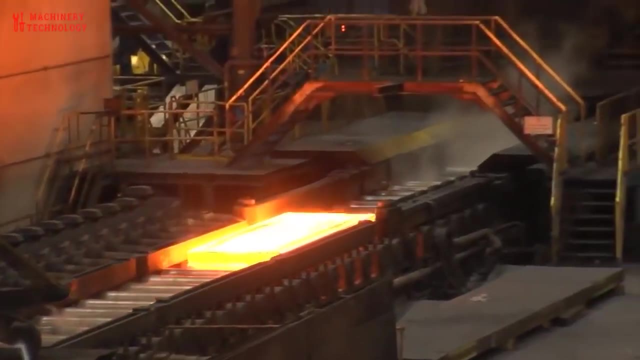 wanted dimensions. Then steel sheets are spun until coiled and left to cool. For bars and a beam steel is sanctioned and cooled. Hot rolling doesn't give precise dimensions, since steel shrinks while cooled. so the resulting steel is suitable for applications where minutely specific dimensions aren't crucial, like 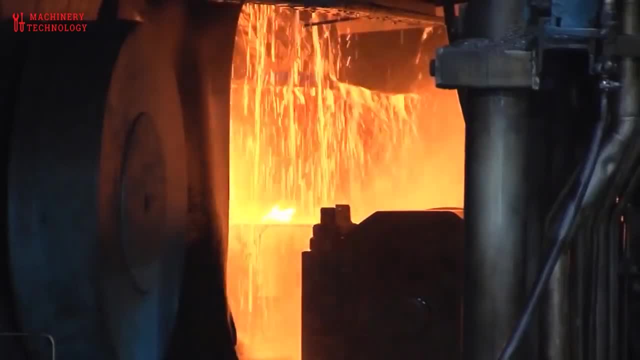 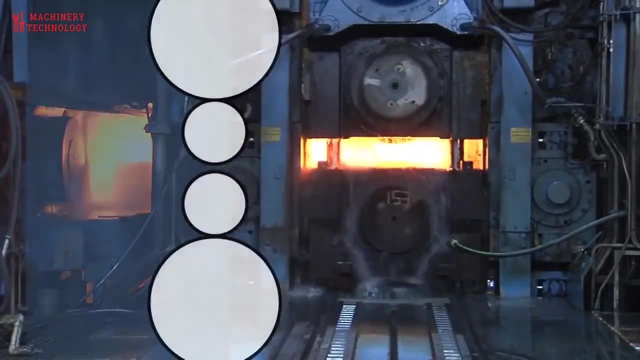 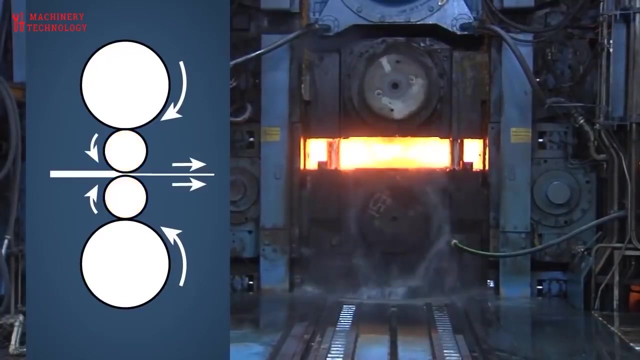 railroads and constructions. Hot rolling steel can be defined by these features due to the shrinking remnant of cooling, A scaled surface, slightly rounded edges and corners or slight distortions. advantages of hot rolling steel: Cost efficiency, because it's required much less processing with a cold rolled steel. 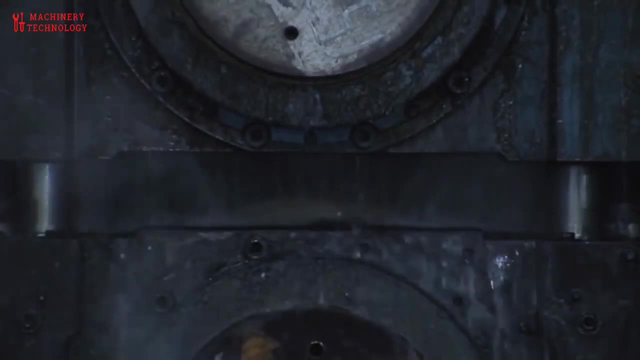 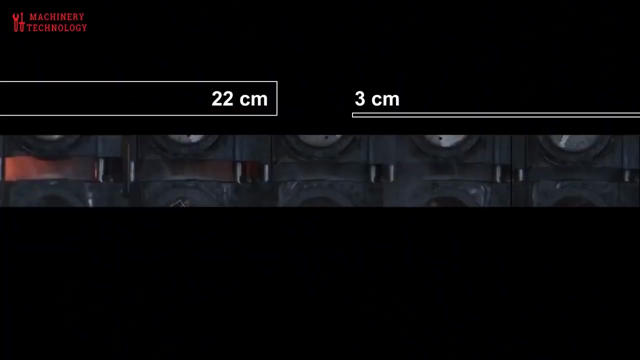 Fee from internal stress that arise while cooling, since it's left to cool at room temperature. Ideal for application where accurate dimensions are not important at all. Hot rolled coils. Hot rolled coils are one of the flat steel products. They are sheets of prime or second choice steel that are rolled in a hot steel mill. 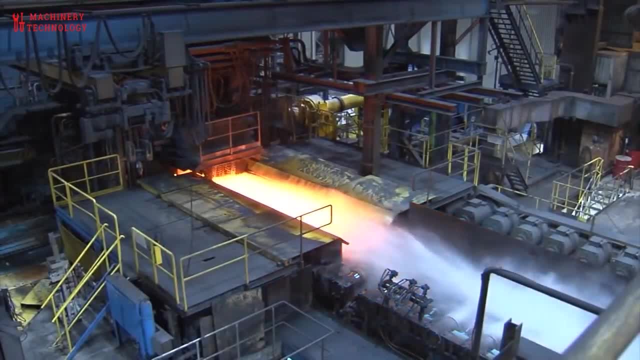 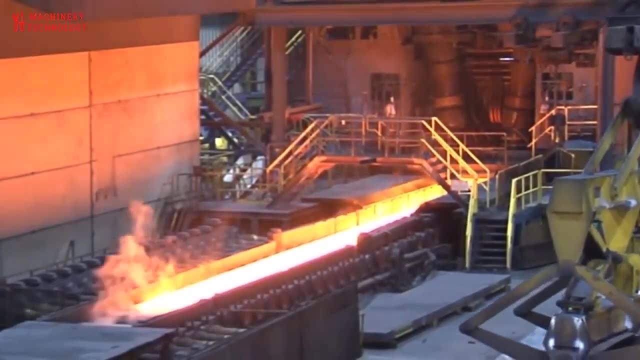 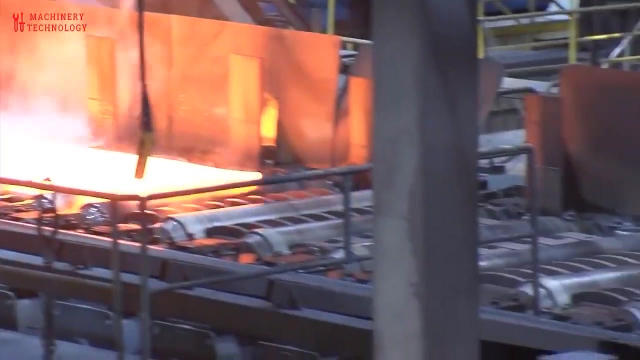 into coils while they are very hot. These coils are very common types of steel coils that form the base product for other steel coils, like coated and galvanized coils, and also used directly nearly in various industries and machinery, Like construction, shield welding, auto car industry, etc. 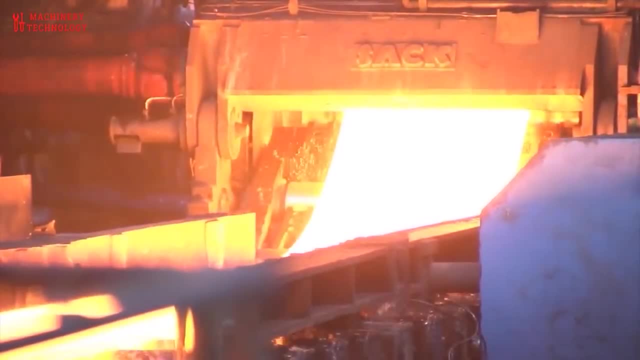 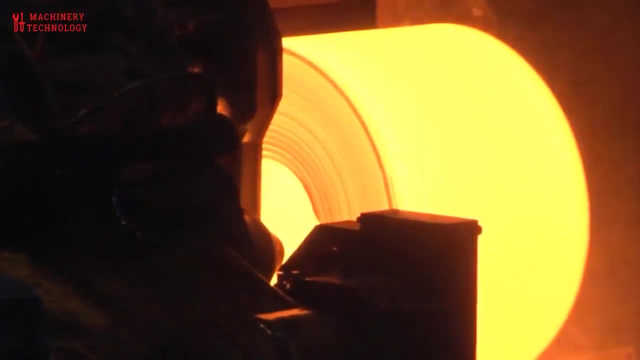 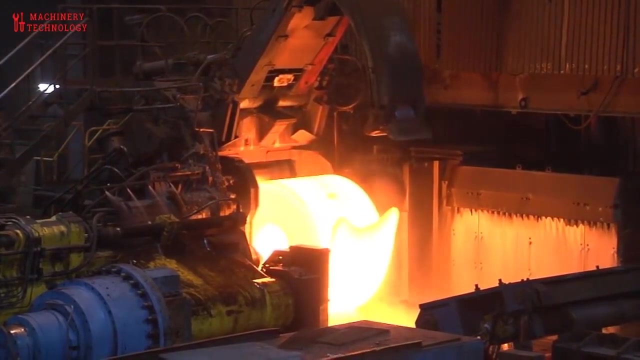 Hot rolled coils are a good choice when tide tolerances are not so important and when price is more important than precision. They are a preference for steel companies and metalworking due to their malleability and cost efficiency. Hot rolled coils have an appearance that distinguishes them over their old coil types. 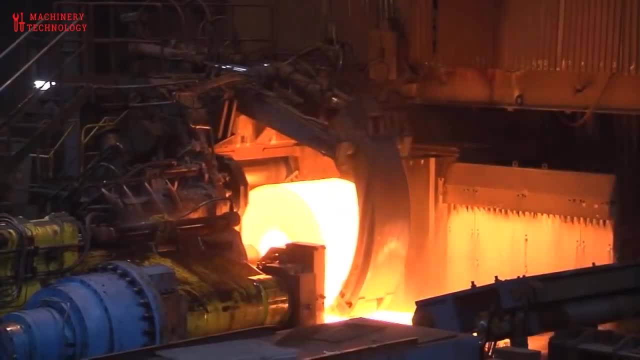 They are darker gray and have a silvery blue, almost purple strip along both sides. They are also a good choice when tight tolerances are not so important and when price is more important than precision. They are a preference for steel companies and metalworking due to their malleability and. 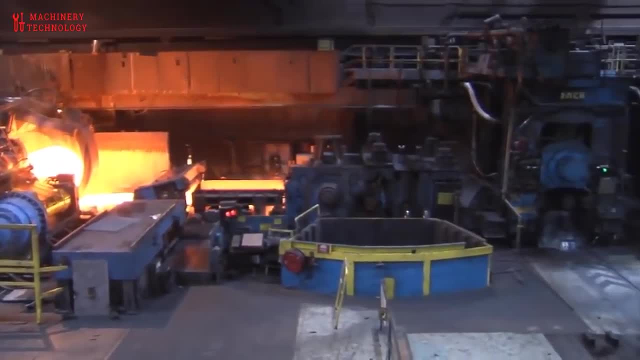 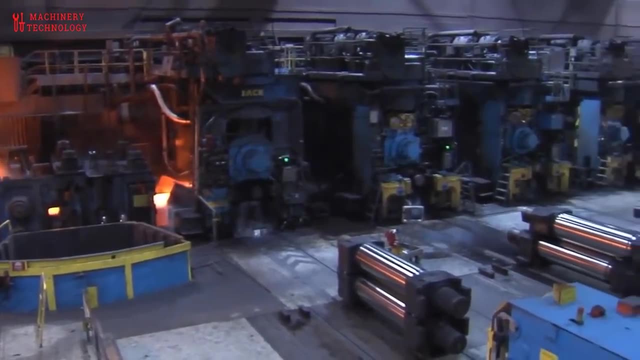 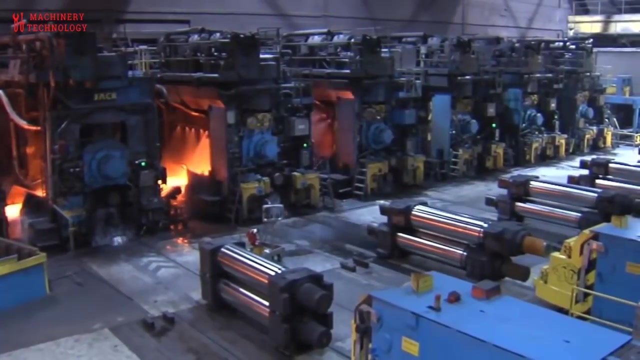 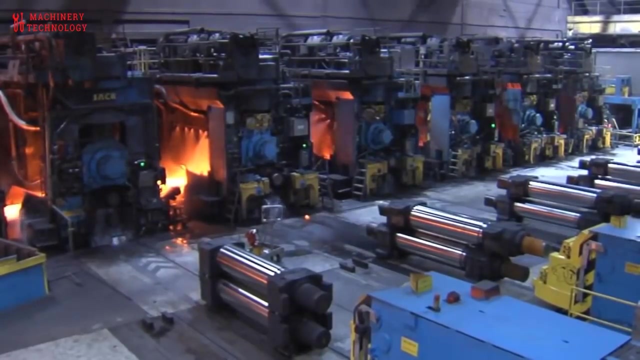 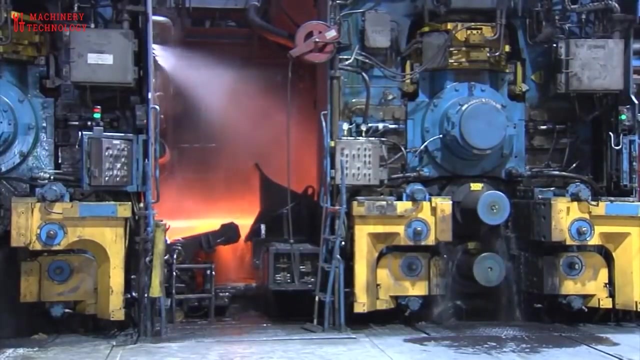 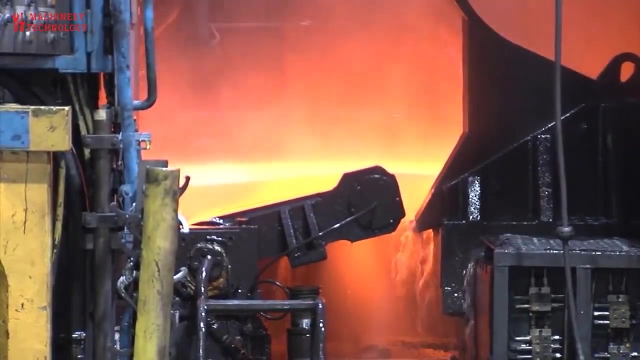 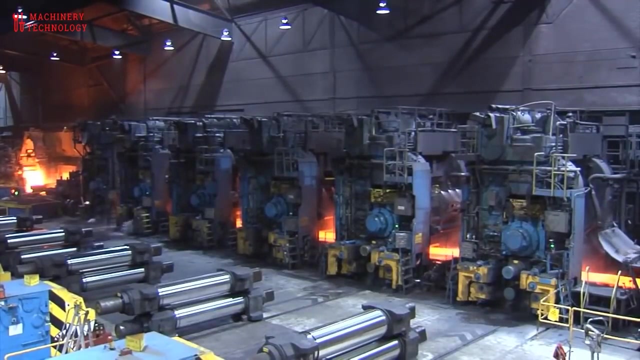 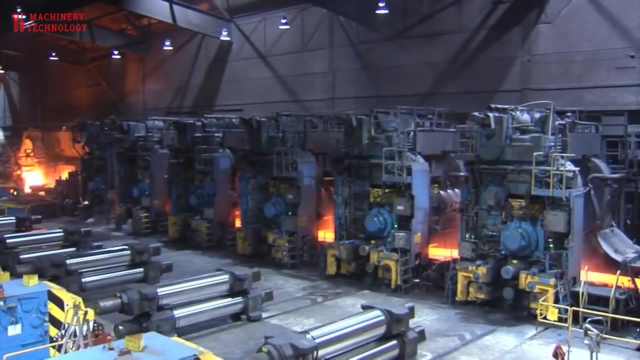 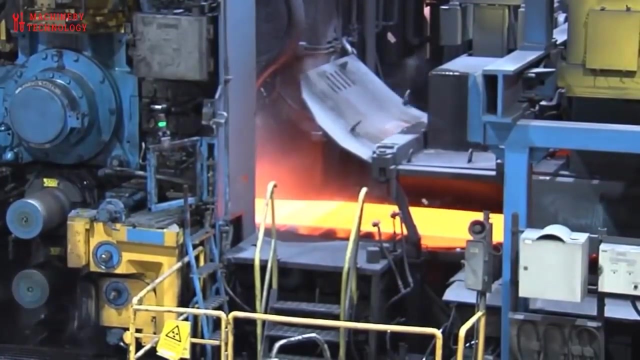 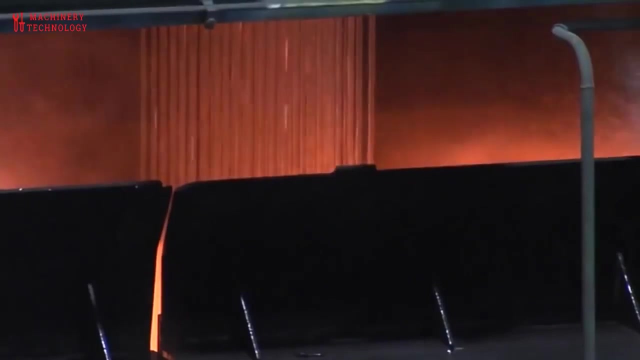 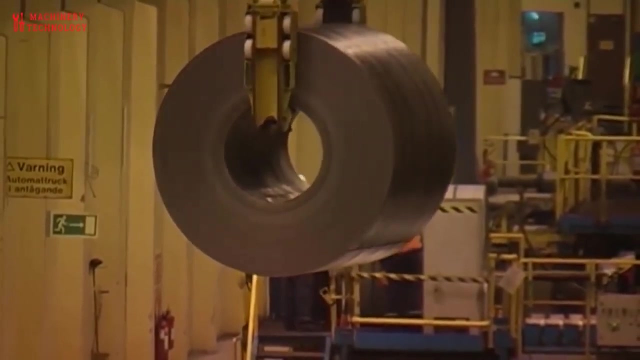 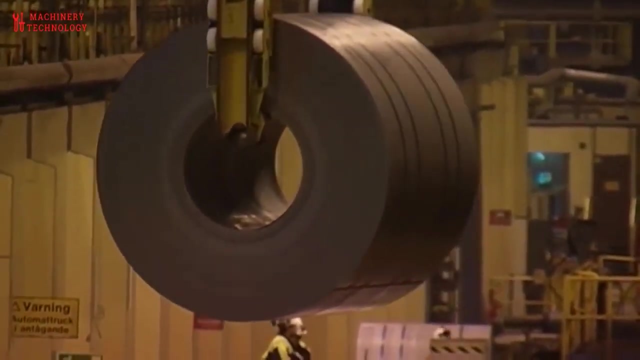 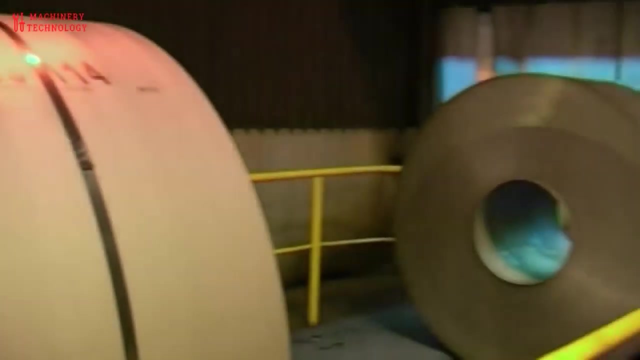 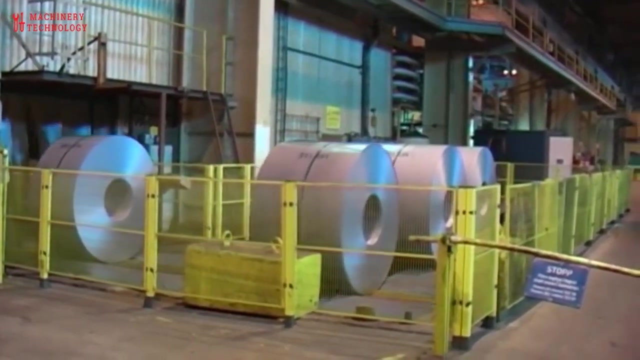 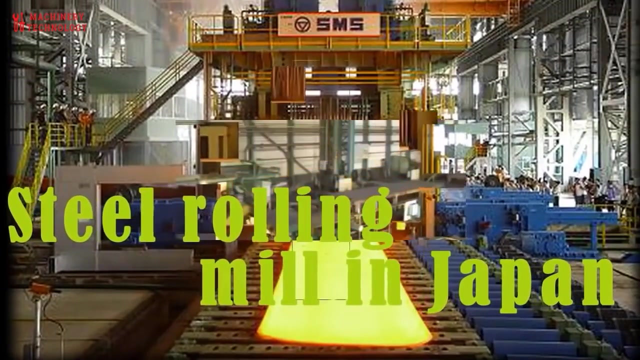 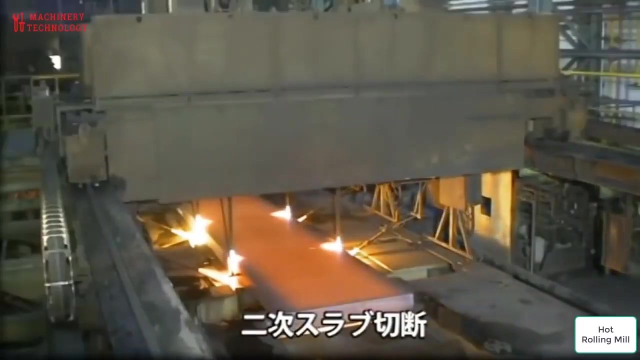 cost efficiency, As the long both sides make the steel surface appear as if it is still hot to the touch. the appearance makes hot-rolled coils the most commonly used type of art sculptures. 入 investment ビ. Thank you, Thank you, Thank you. 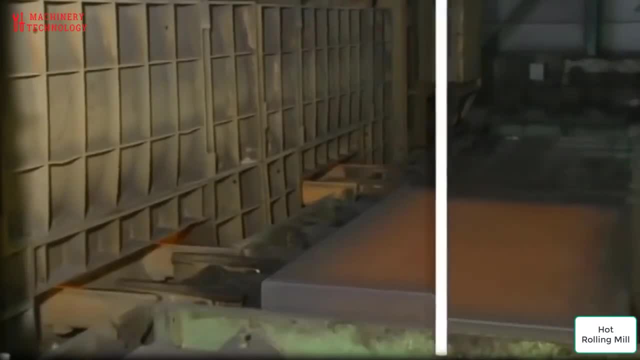 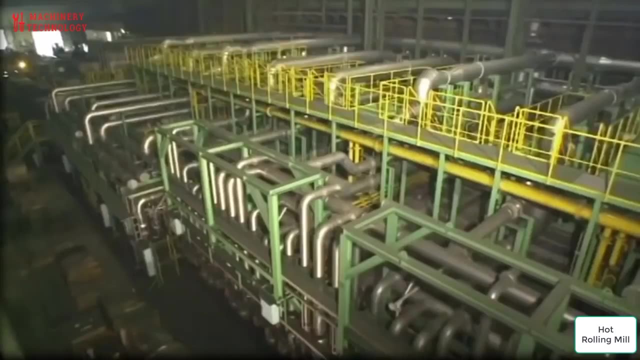 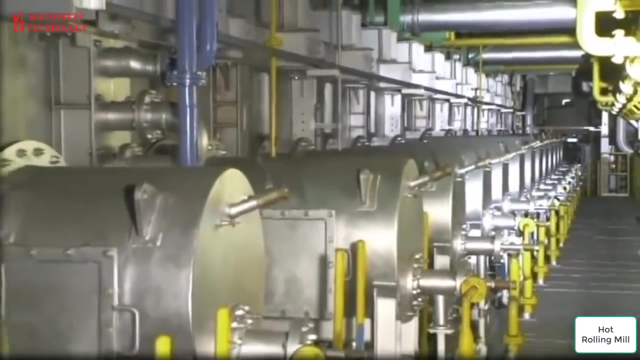 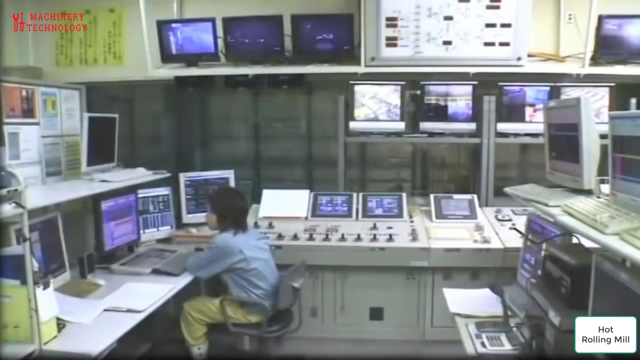 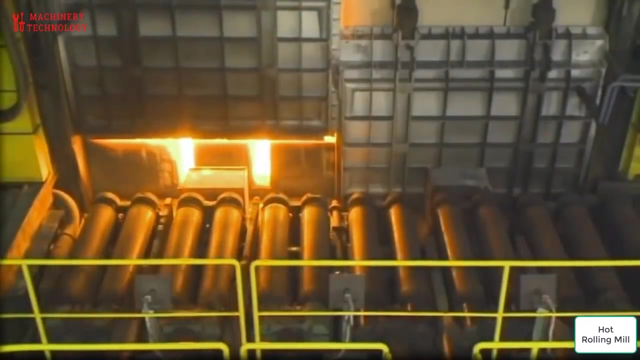 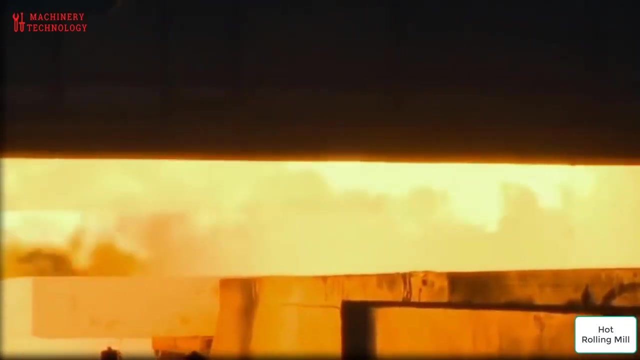 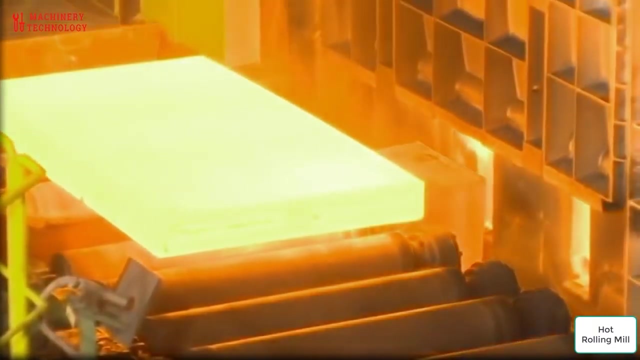 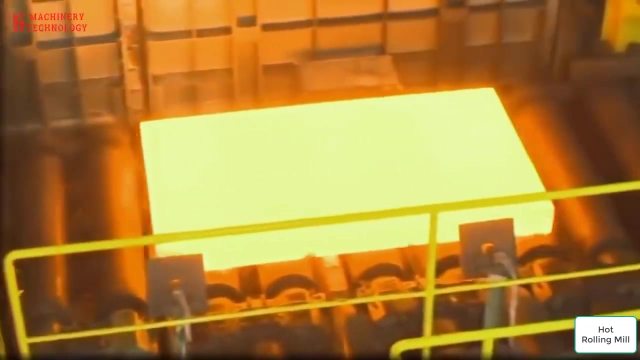 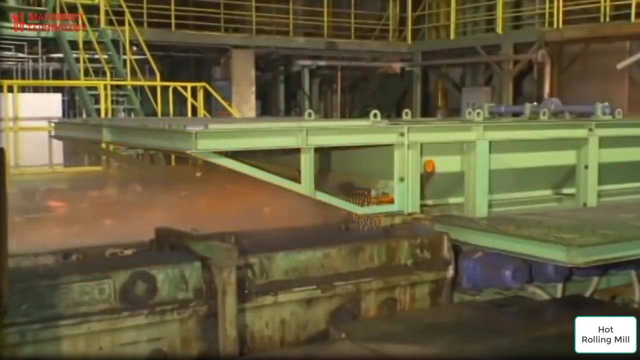 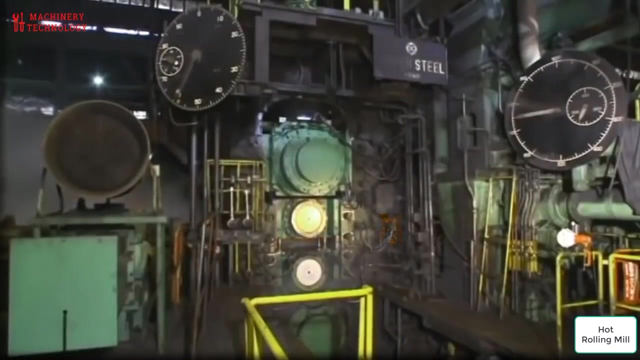 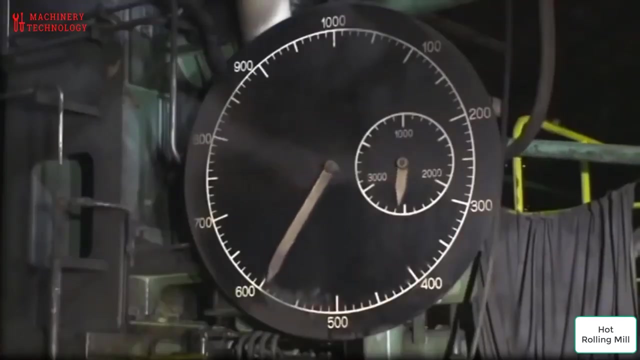 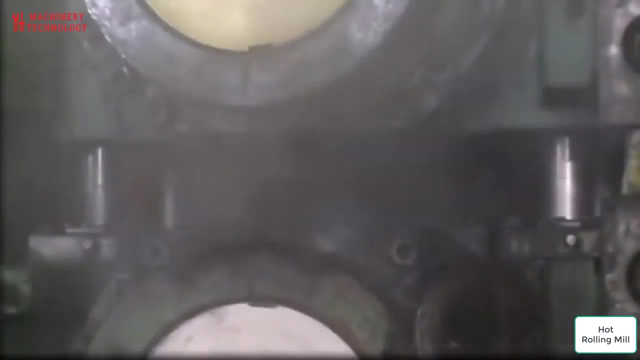 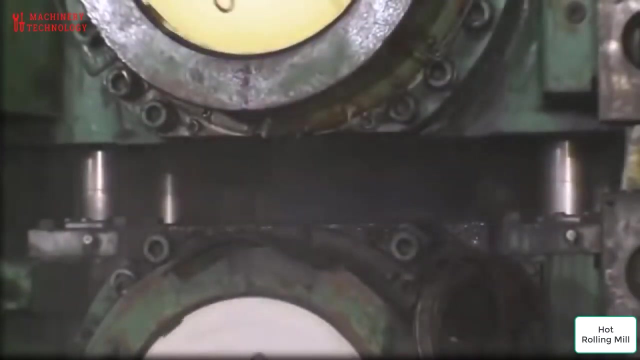 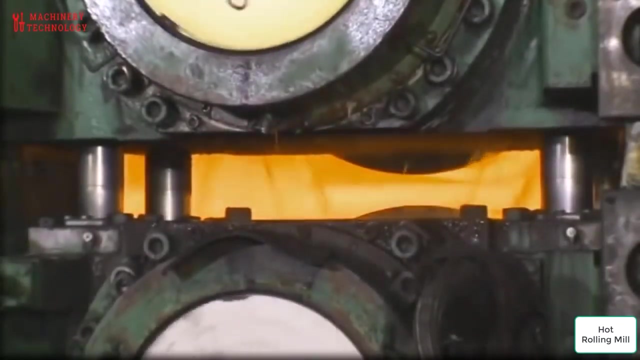 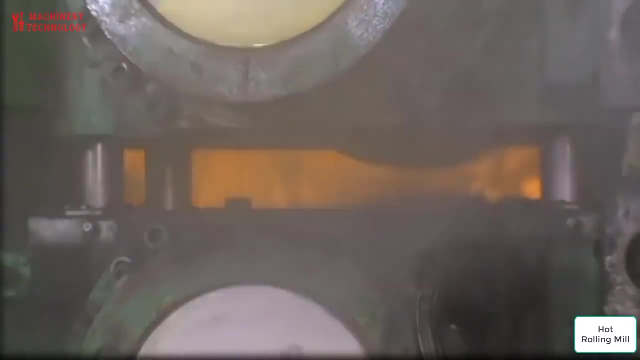 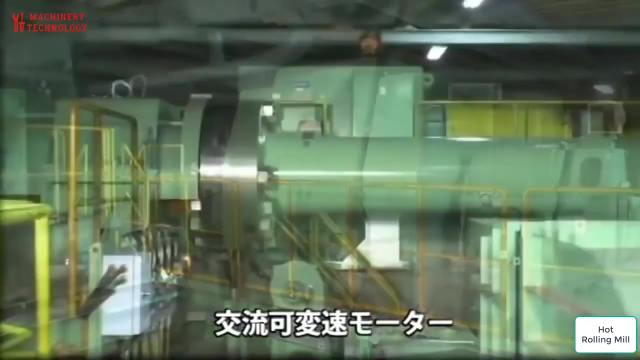 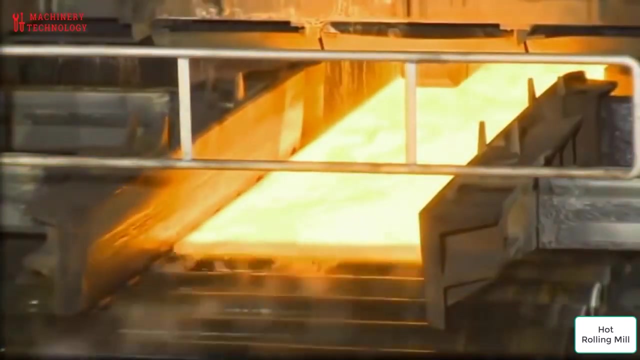 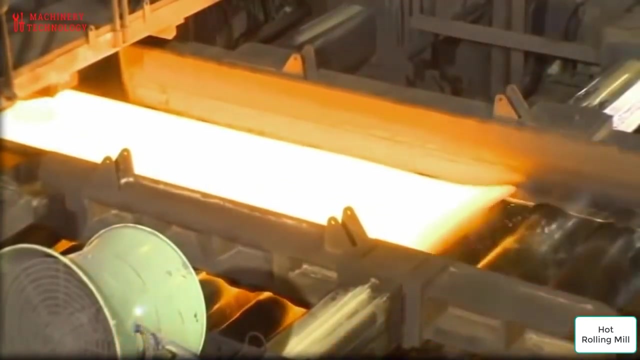 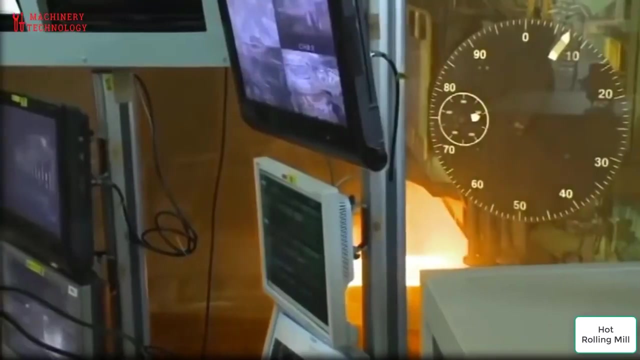 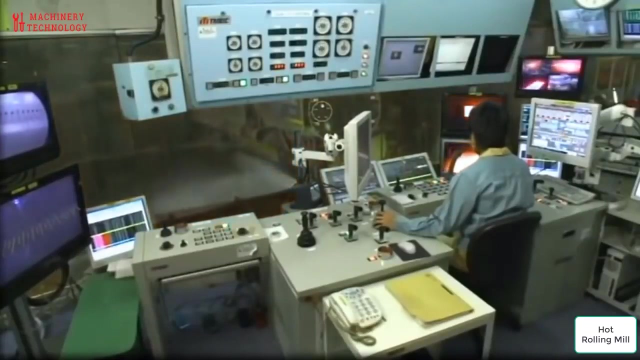 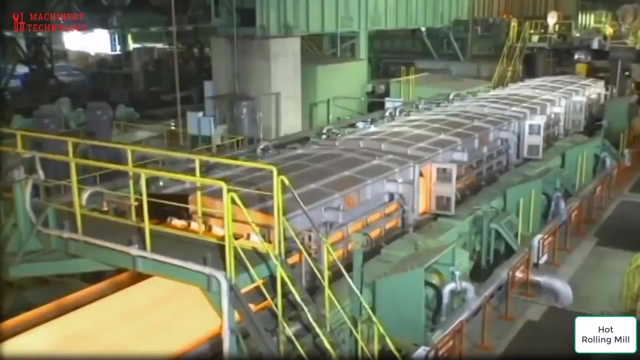 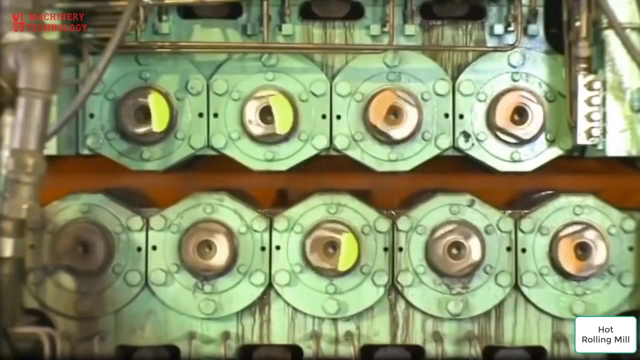 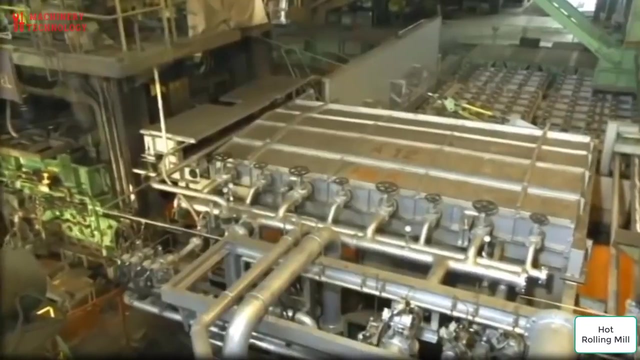 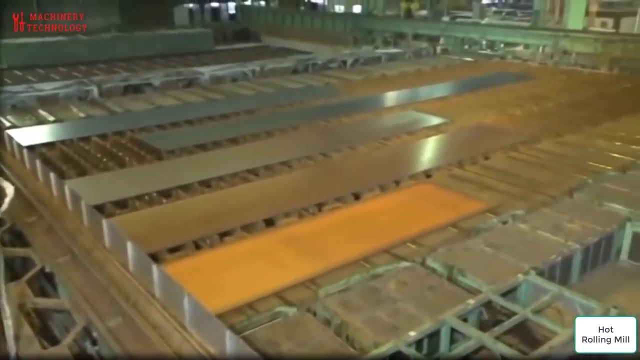 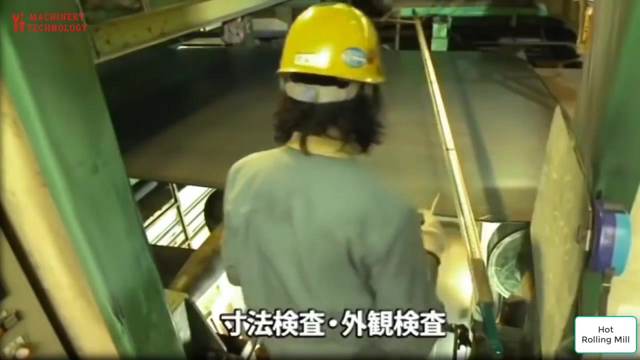 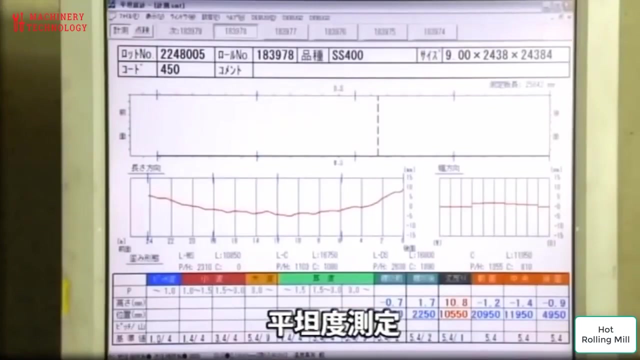 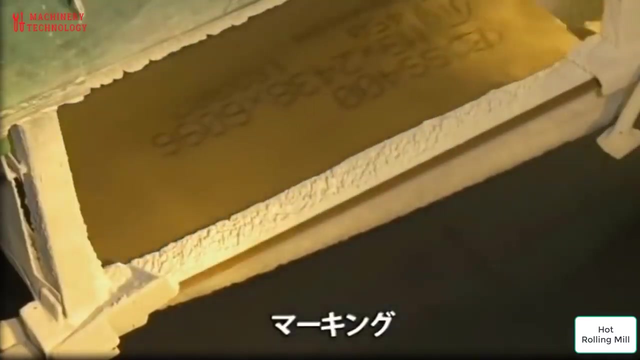 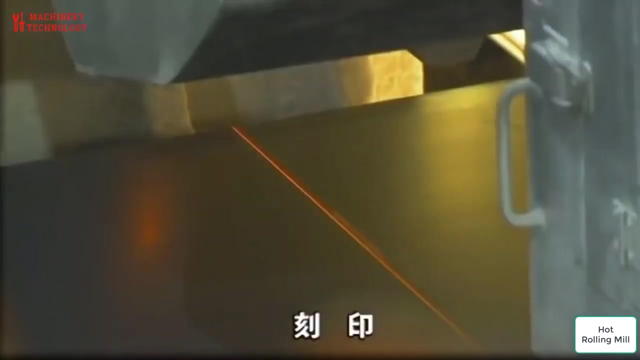 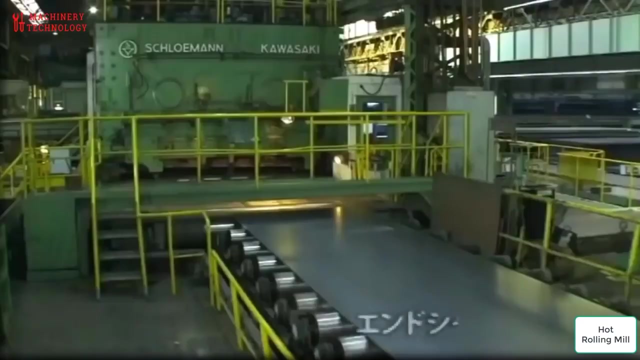 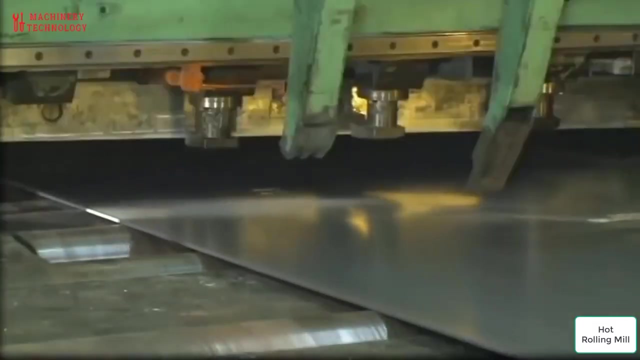 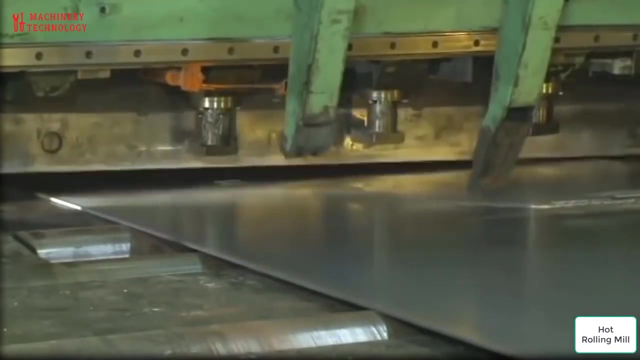 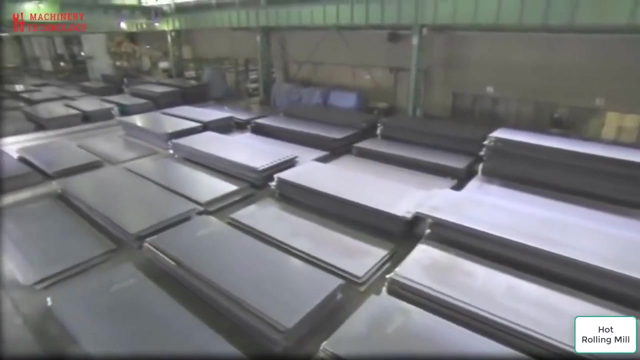